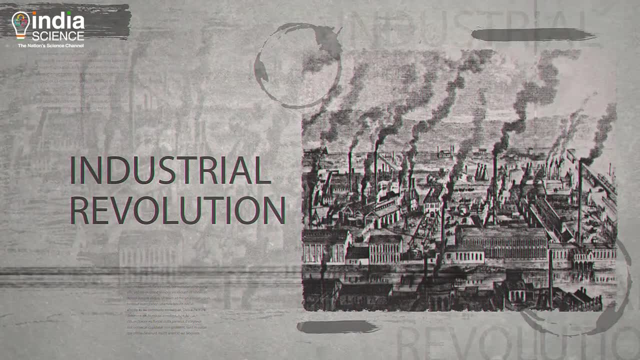 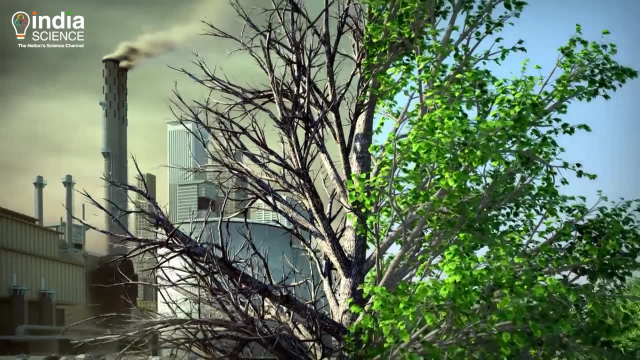 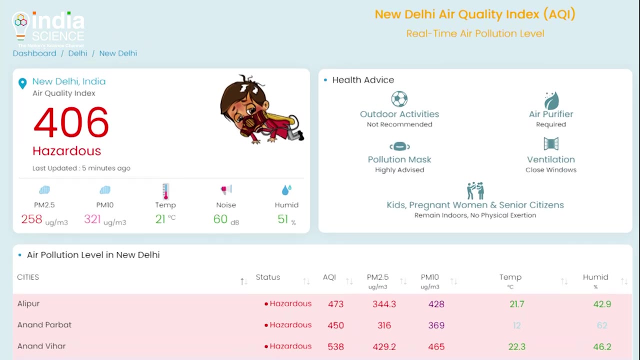 But since the Industrial Revolution in the 1800s, humans have been adding harmful substances into the atmosphere in levels that threaten the environment and human health. Your city's air quality is measured using the Air Quality Index or the AQI. AQI provides a score that ranges from 0 to 500,. 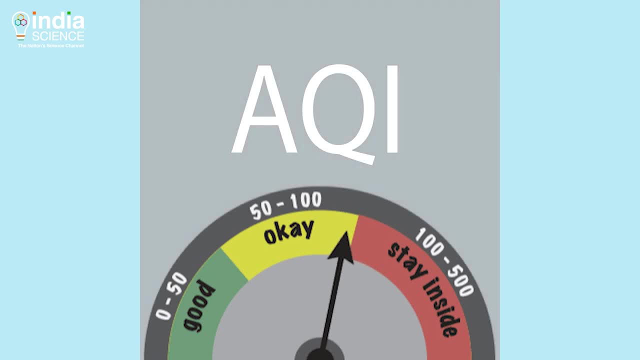 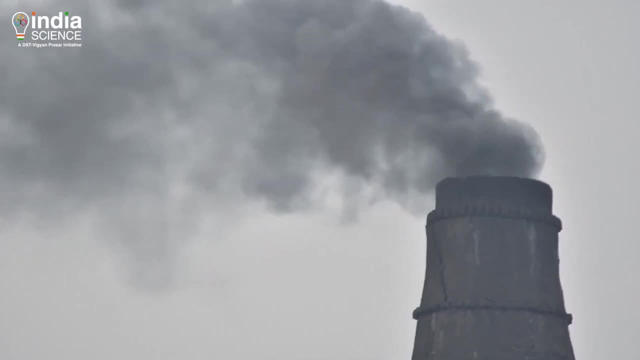 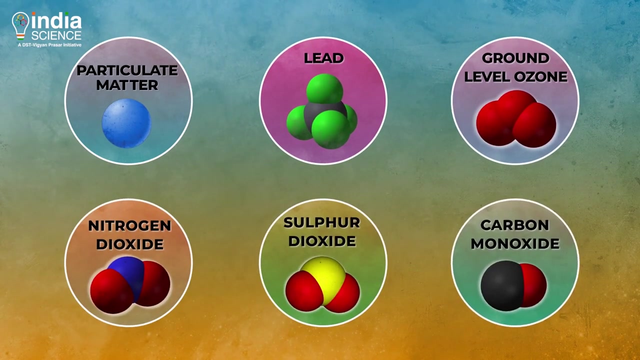 with 0 being the safest and 500 the most hazardous. So how is it calculated? It is done by measuring the atmospheric levels of substances like carbon monoxide, nitrogen dioxide, ozone, sulphur dioxide, particulate matter and the like. 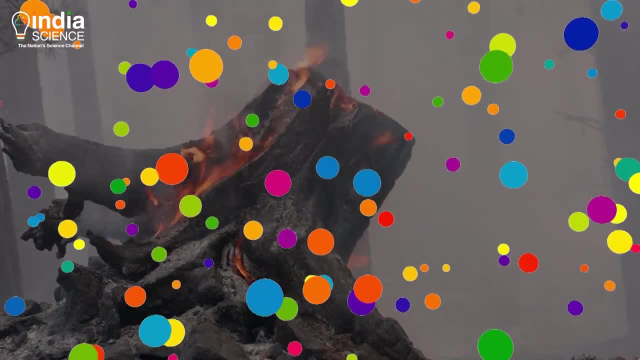 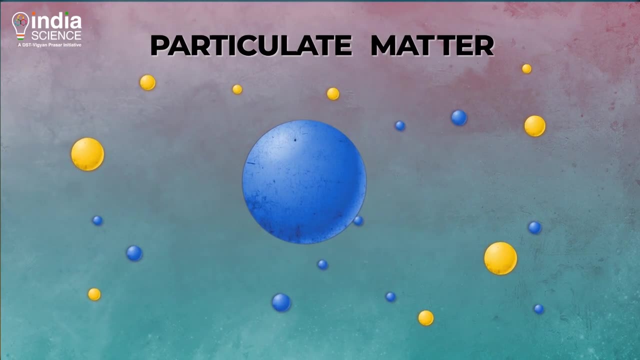 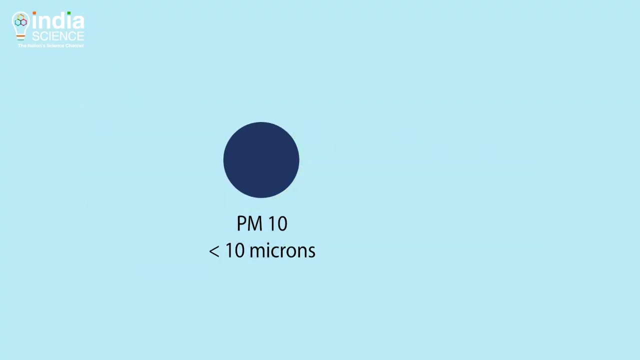 When their levels in the air shoot beyond a certain limit, they become pollutants. Particulate matter is a mixture containing solid particles or liquid droplets released from power plants, fossil and biomass fuels. Some particles could measure 10 micrometres, 2.5 micrometres or even smaller. 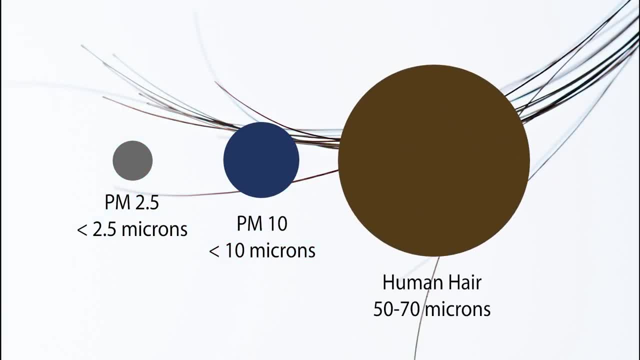 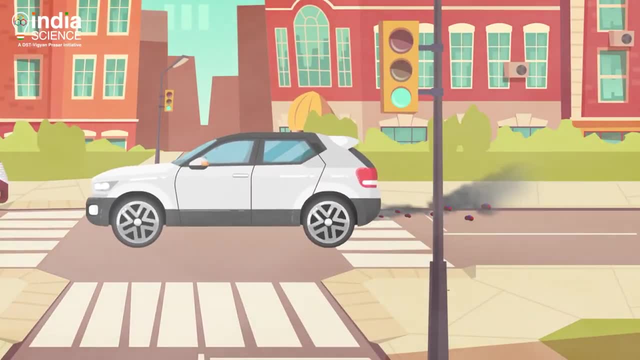 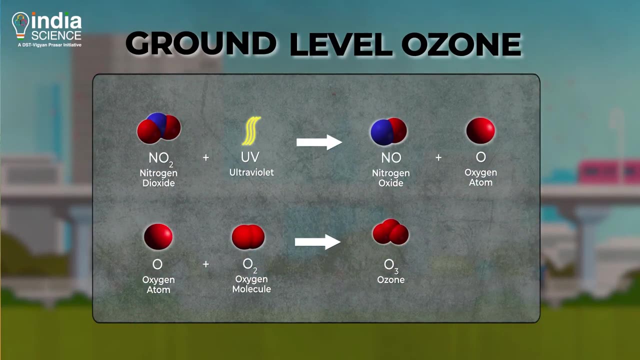 For comparison, a strand of human hair measures 50 to 70 micrometres. Nitrogen dioxide is emitted from vehicles and power plants. Sulphur dioxide escapes from power plants. Ozone is formed when nitrogen dioxide reacts with other substances. 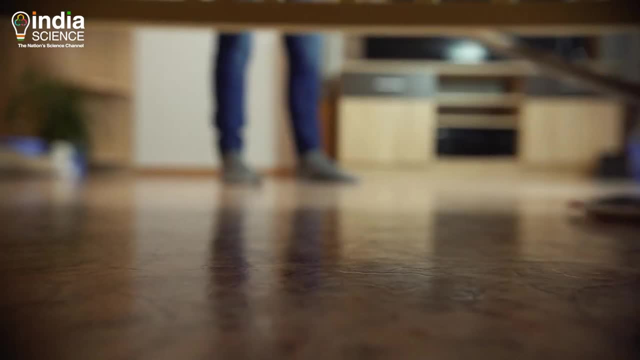 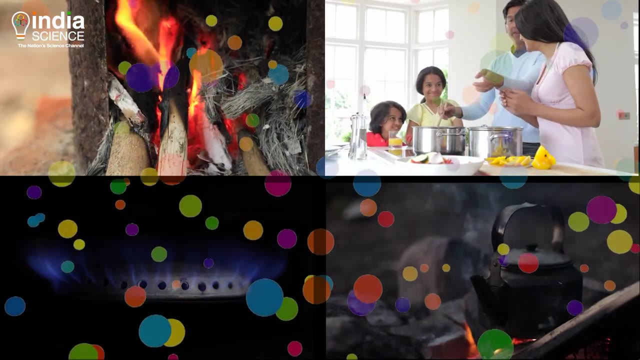 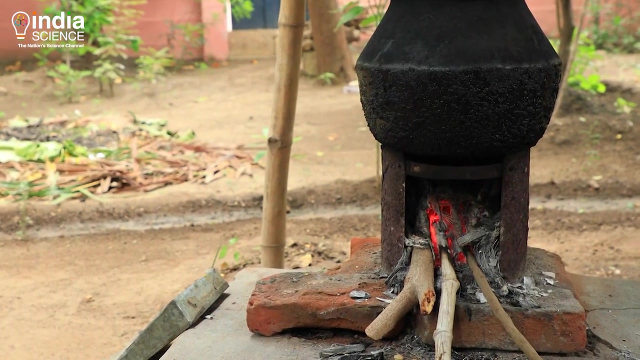 These pollutants could also be hiding in your homes. We tell you how Activities like cooking and heating can give rise to carbon monoxide, nitrogen dioxide and particulate matter. Rural homes are thought to bear the brunt, as they rely on burning biomass fuels. 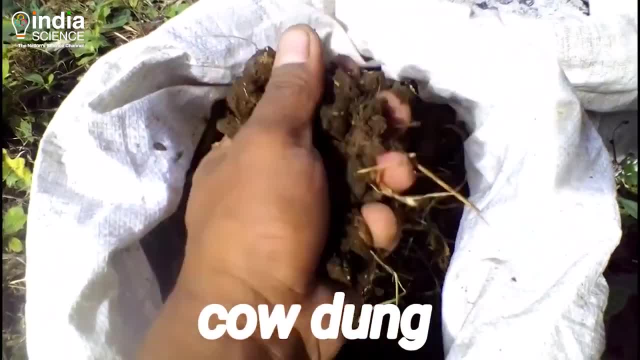 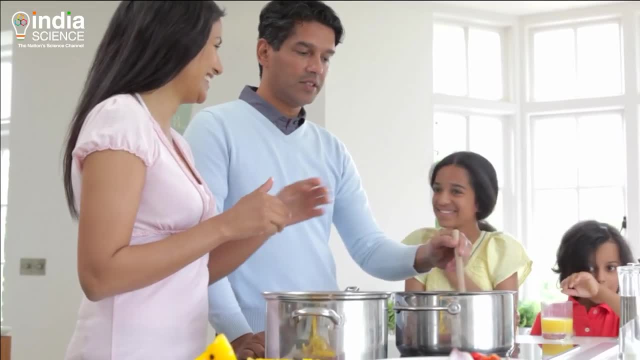 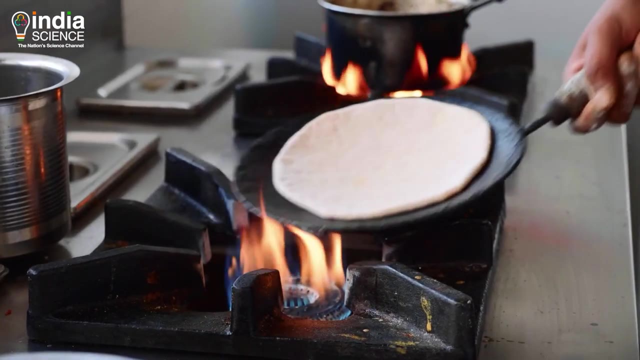 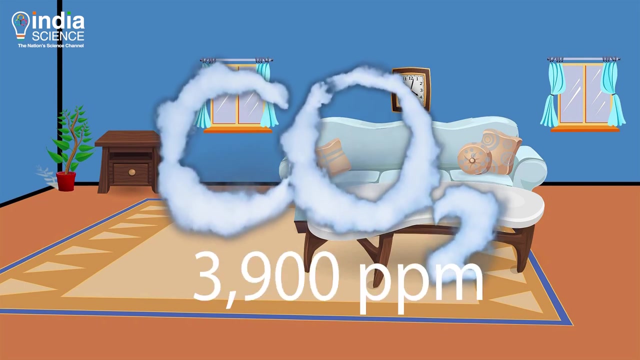 such as wood charcoal and dung for cooking or heating, exposing themselves to harmful gases in the process. This, however, does not mean that urban households are safe. Gas-burning stoves are also believed to emit pollutants. One study found that indoor carbon dioxide levels in Delhi were 3,900 parts per million. 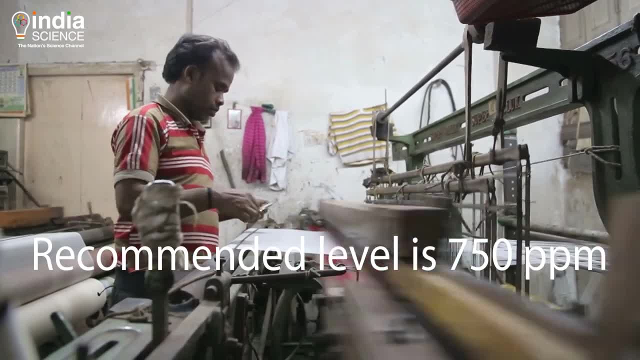 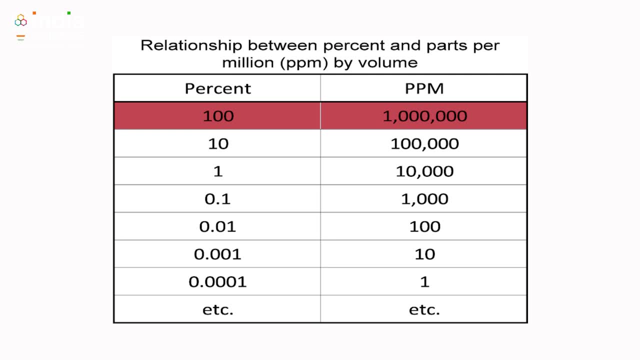 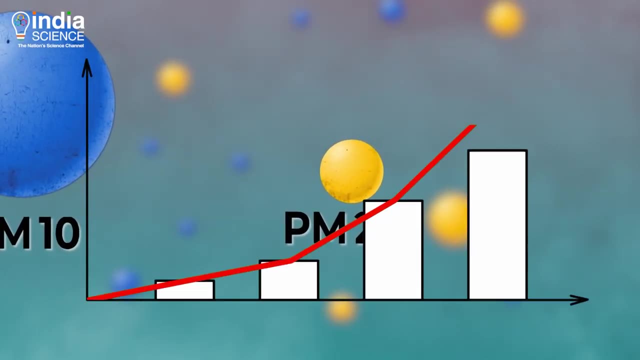 The recommended safe limit is 750 ppm. Parts per million, or ppm means out of a million. This is similar to a percentage which is out of 100.. As for particulate matter 2.5, their levels cross the recommended limits. Indoor ppm 2.5 or particles that measure 2.5 micrometres or lesser. 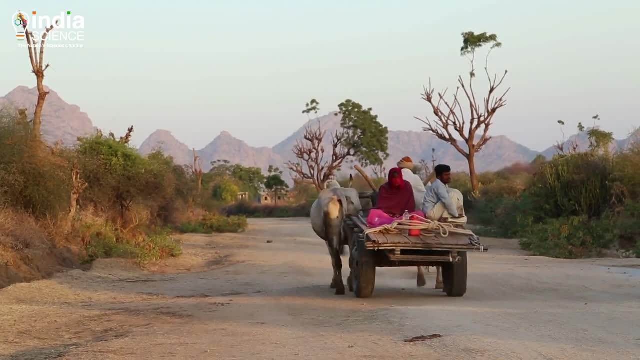 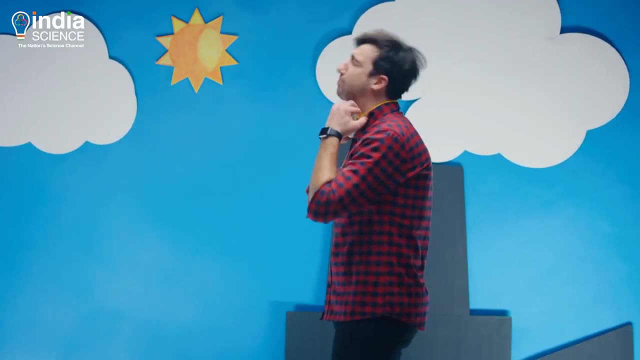 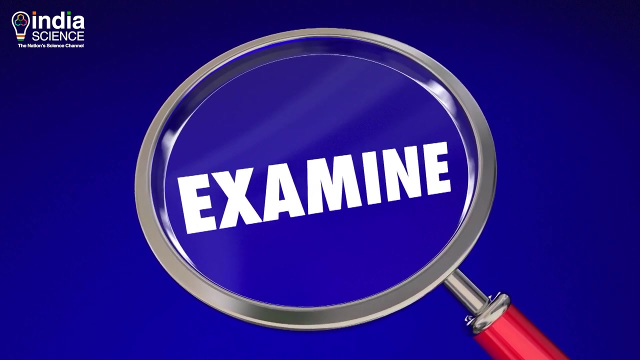 is 10 times more powerful than those found outdoors. This is because indoors are generally closed and contained. So what do these pollutants do to your body? Before we look at ppm 2.5, let's examine the other notorious gases: Nitrogen dioxide and carbon monoxide. 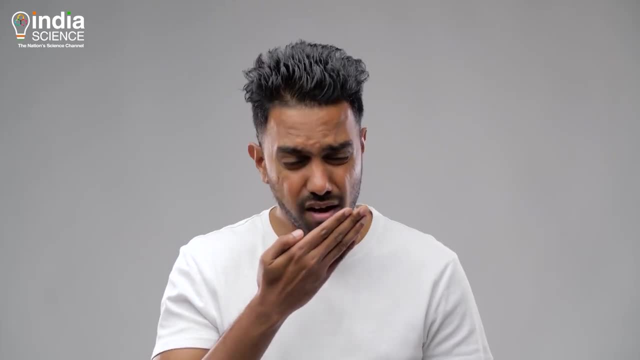 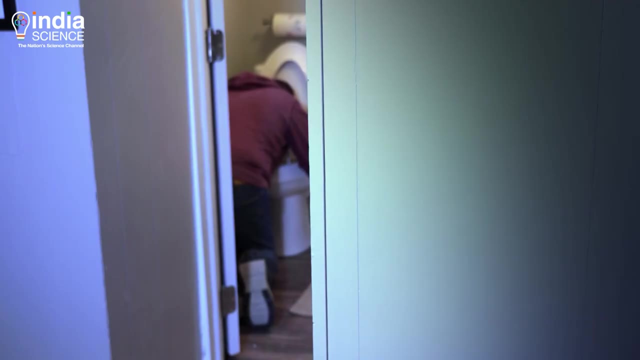 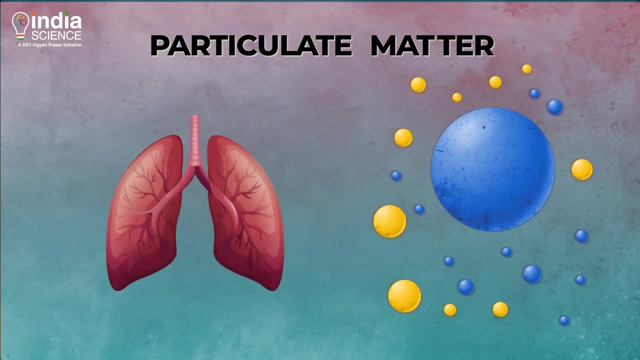 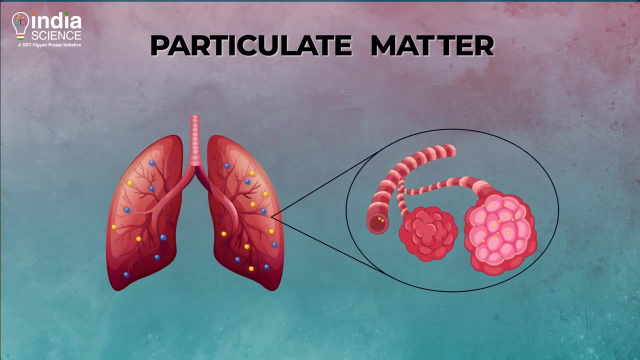 Upon inhaling them, you might experience coughing, sneezing and breathing problems. Carbon monoxide poisoning can lead to headache, nausea, a rapid heartbeat, cardiac arrest and even death. Particulate matter 2.5 is particularly dangerous because they can infiltrate the deepest parts of your lungs. 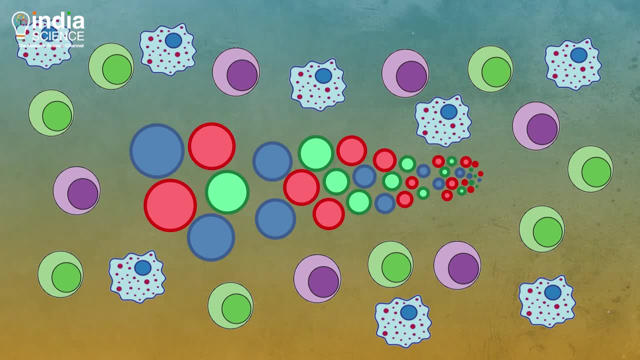 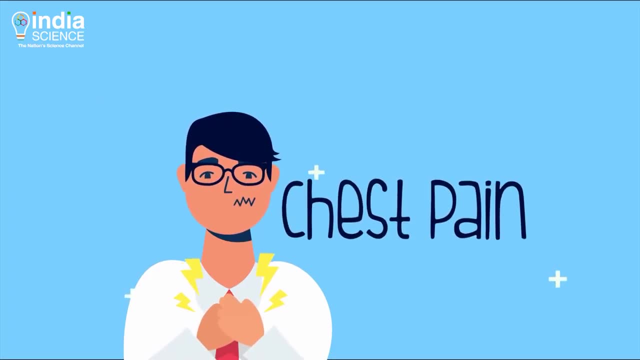 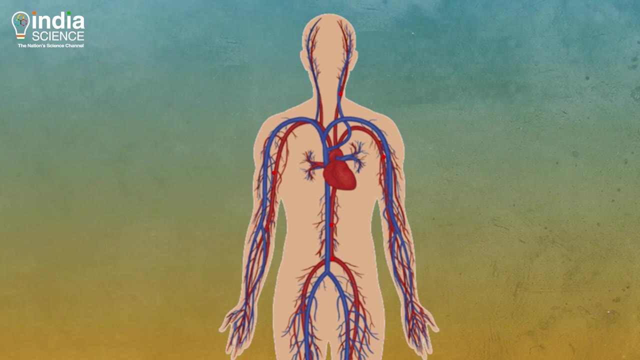 In response, our immune cells surround the pollutant and release molecules that cause inflammation, And inflammation leads to chest pain and breathing problems. From the lungs, these particles are carried to other parts of the body through the bloodstream. ppm 2.5 may also cause heart diseases in the long term. 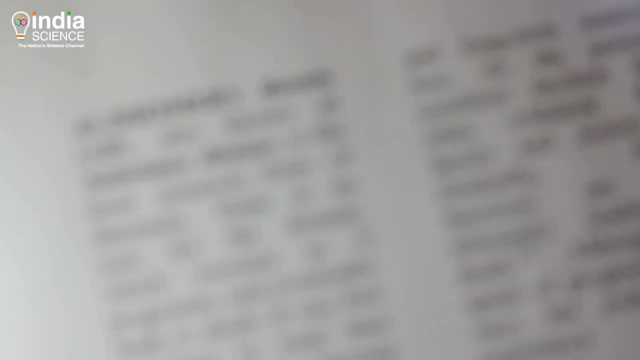 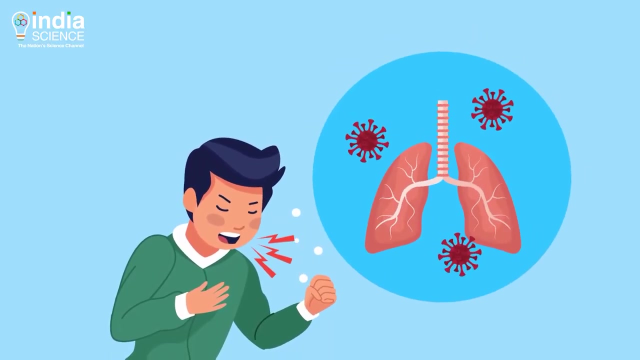 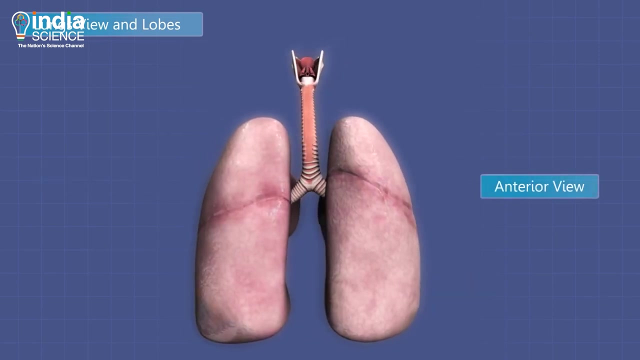 It does not spare the brain either. These fine particles appear to lead to Alzheimer's disease. They could worsen infectious diseases like COVID-19.. They could cut lives short. Children have a narrow airway, making them more vulnerable to the damaging effects of air pollution. 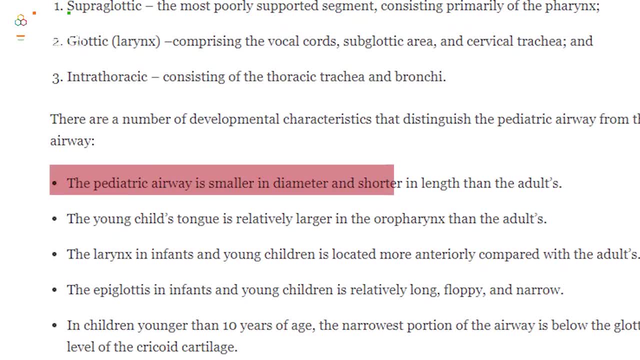 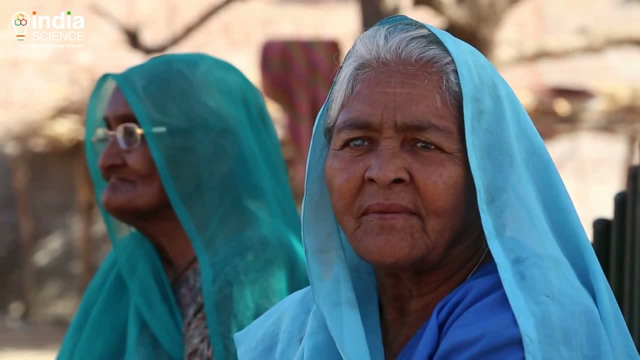 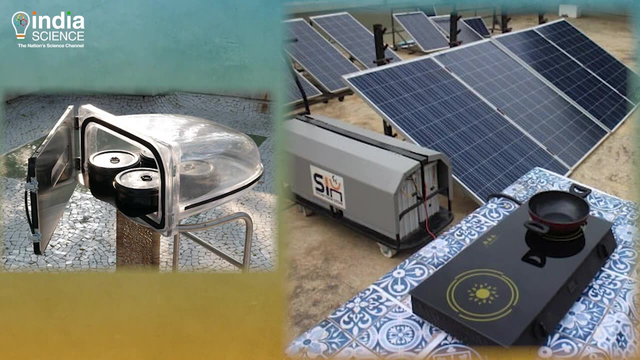 It is smaller in length and diameter than the airway found in adults. Women and elderly are also at risk because they spend more time indoors. But is it possible to keep the air in our homes cleaner? Yes, it is. You could adopt solar stoves. 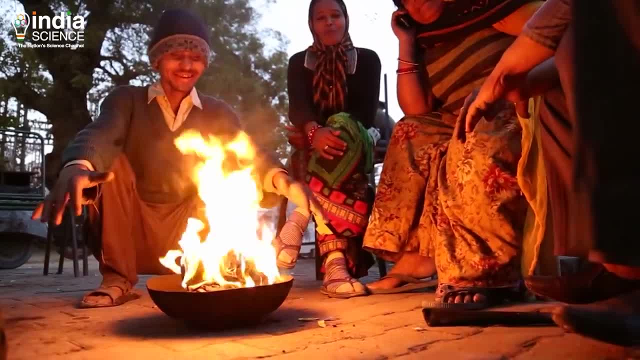 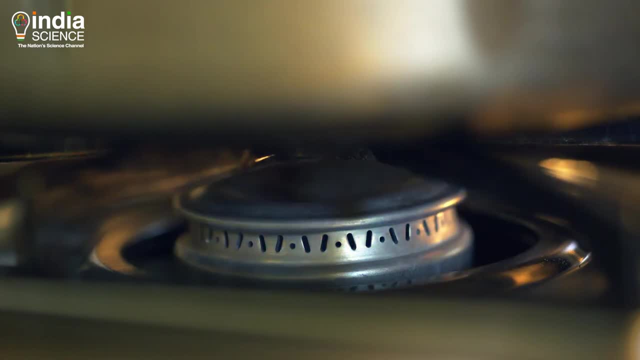 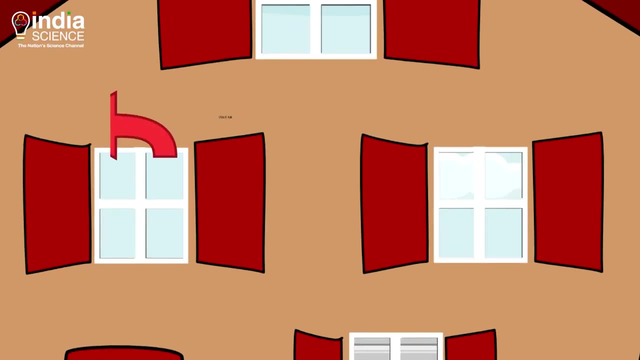 It is the cleanest form of energy. Solar stoves could especially help rural households that depend on biomass fuels. You could also consider replacing LPG with electric stoves. The other solution is allowing good ventilation. This allows the exchange of stale and fresh air. 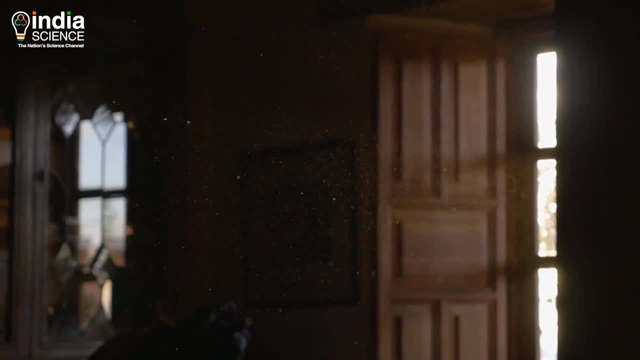 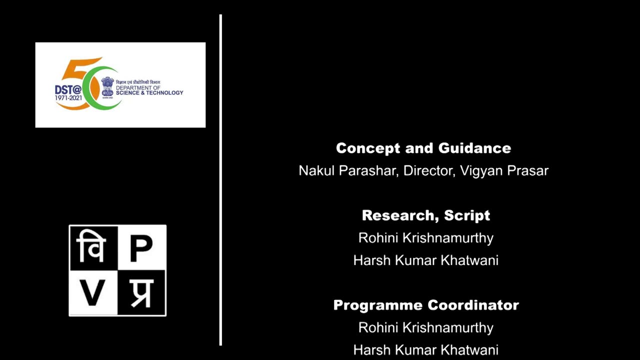 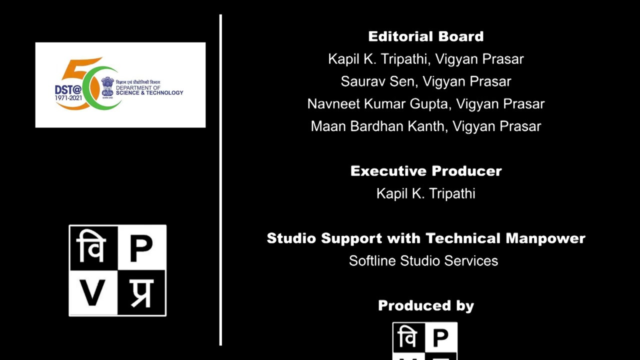 So every time you cook, remember to keep your windows open. This is the solution for the most vulnerable people in the world. You can also purchase a solar stoves in a store. For more information, visit us at wwwncdcca. For more information, visit us at wwwncdcca. 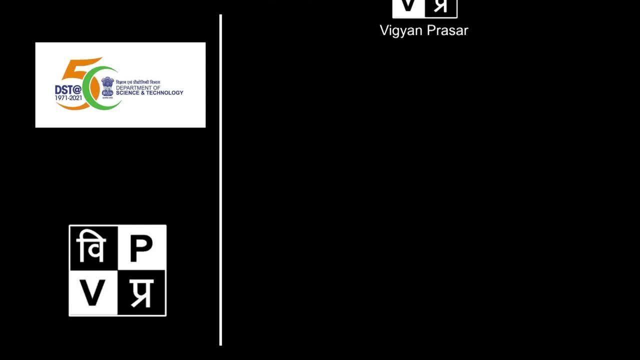 For more information, visit wwwncdcca. For more information, visit us at wwwncdcca.